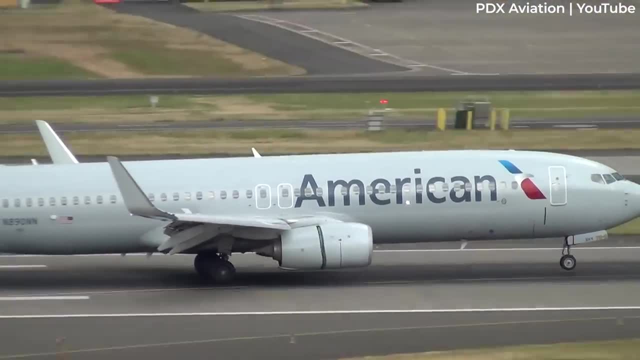 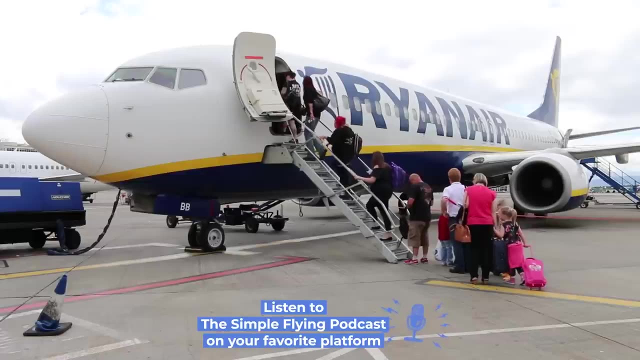 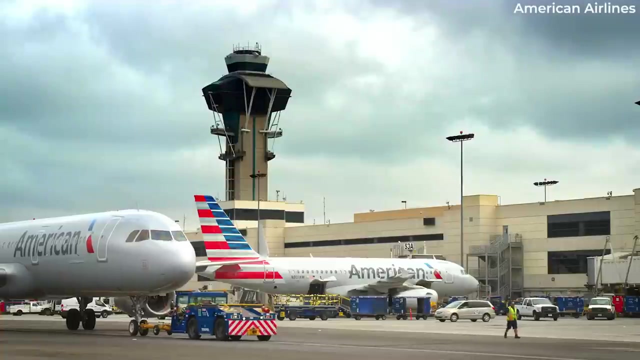 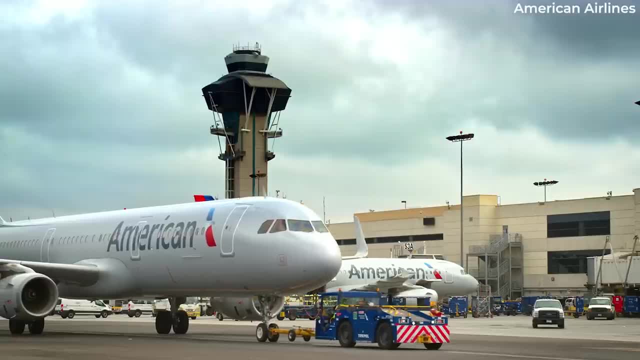 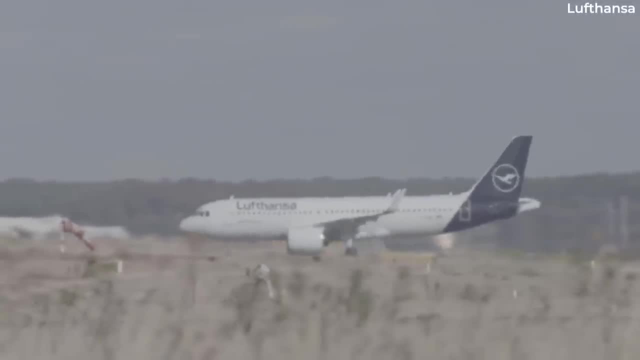 The A320CO in 737-800 have been excellent choices for balancing trip cost, seat mile cost and not having too many seats to fill. Obviously, these narrowbody jets are increasingly superseded by aircraft with more modern technology with far lower fuel burn. Aircraft like the A320neo, which ranked 7th globally in 2022,, and 737 MAX 8 in 8th place. However, these are much more expensive to acquire and therefore need greater use to reduce the ownership costs per seat mile. 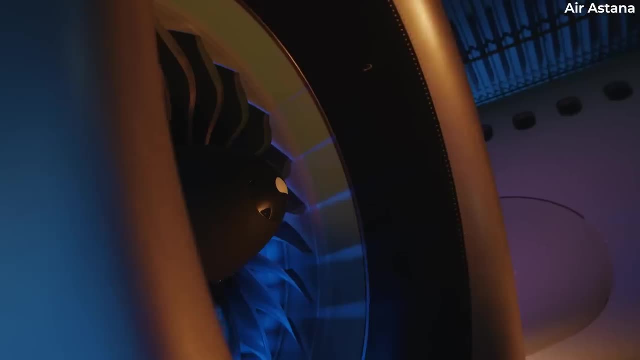 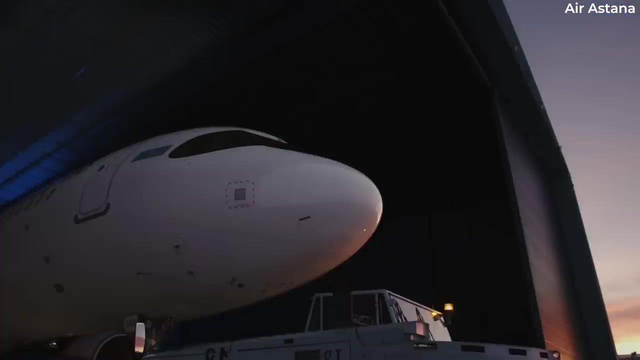 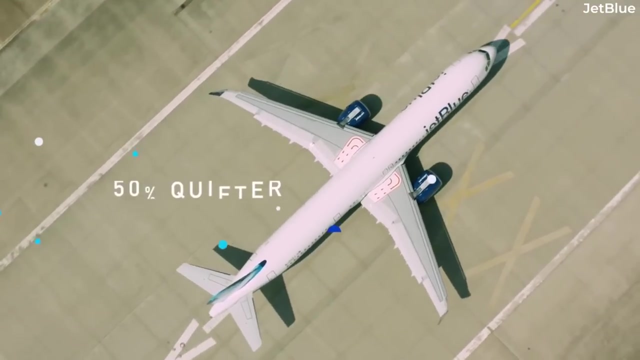 The increasingly popular large narrowbody, the A321neo, with even better economics if the capacity is utilized, fell just outside the top 10, with 609,000 flights. Undoubtedly it will make an appearance on this chart in the future. 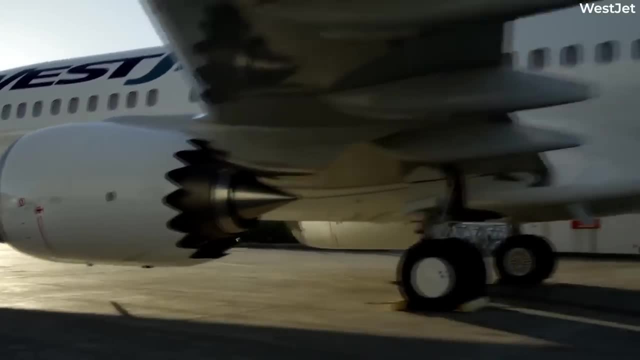 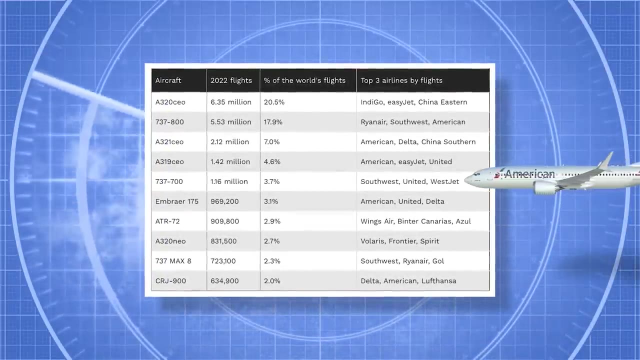 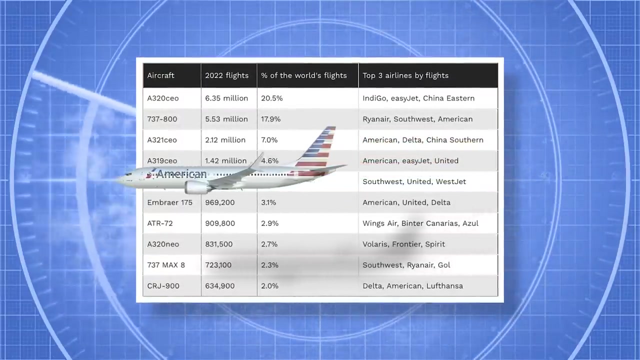 Despite all the problems afflicting the MAX, the MAX 8 managed to make the most used list. After being grounded, American Airlines was the first airline in the US to restart 737 MAX flights following the FAA's recertification of the aircraft. Flight AA718 took off from: 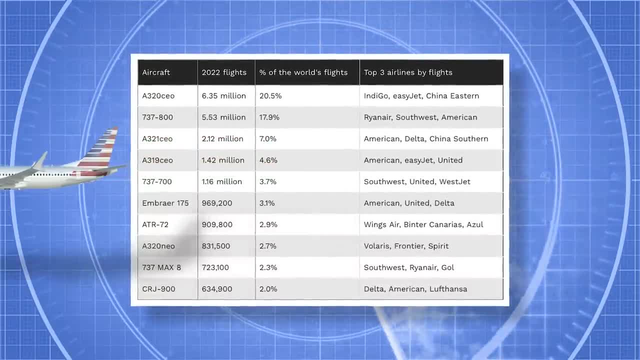 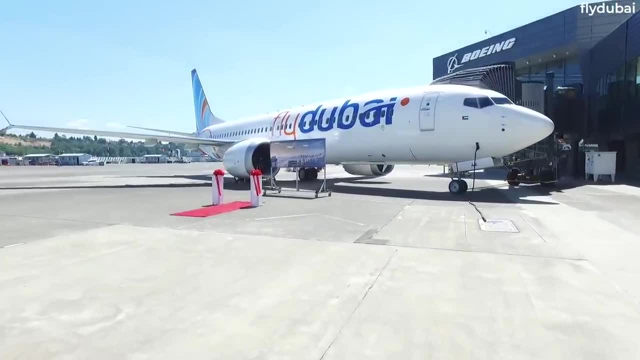 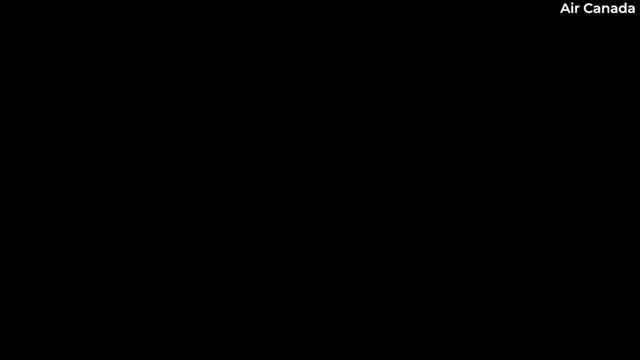 Miami to New York LaGuardia on December 29, 2020, a little over two years ago. Analyzing Sirium data reveals that 708 airports globally had at least 20 MAX 8 flights in 2022.. Not surprisingly, the A321neo is one of the most popular aircraft in the world, with 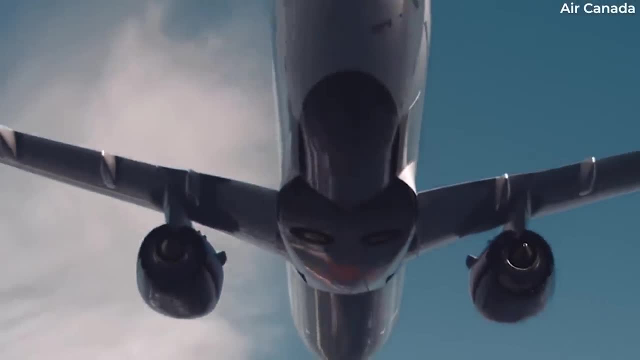 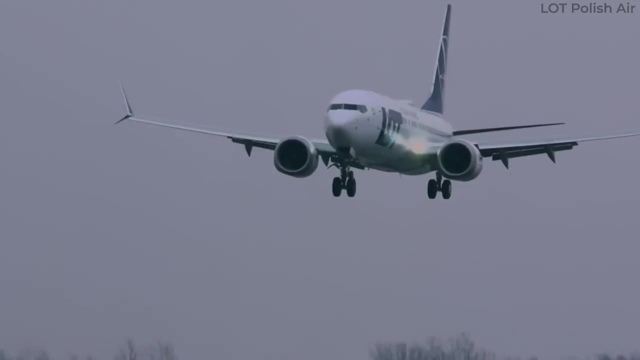 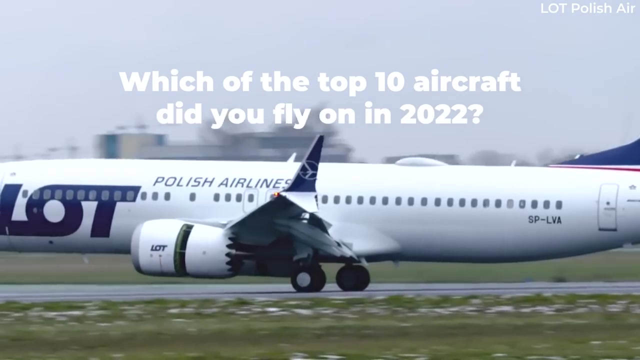 only Miami had the most, followed by Dubai, Mexico City, Vancouver, Toronto, Istanbul Airport, Milan-Bergamo, Honolulu, Las Vegas and Sao Paulo-Guarulhos. How many of the top 10 aircraft mentioned in this video did you fly on in 2022?? Let? 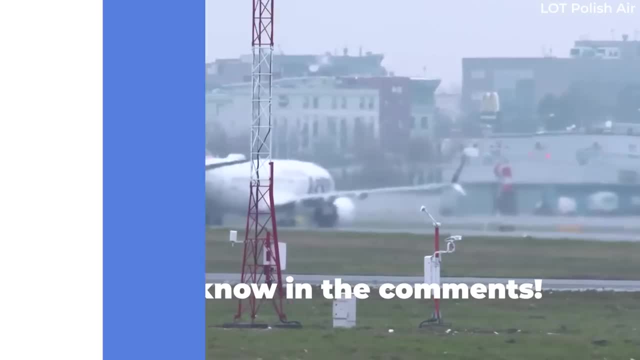 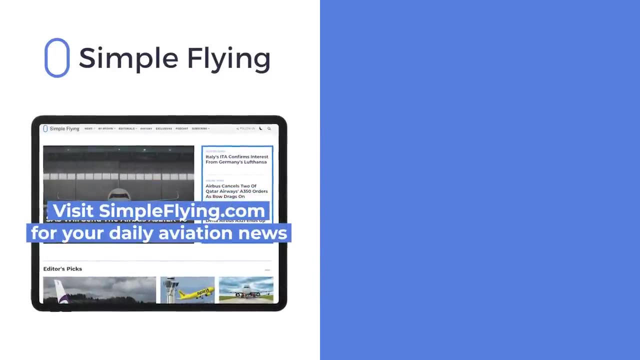 us know in the comments. In addition to our daily YouTube videos, Simple Flying publishes over 150 articles every week. If you are looking for the latest aviation news and insights, visit simpleflyingcom.